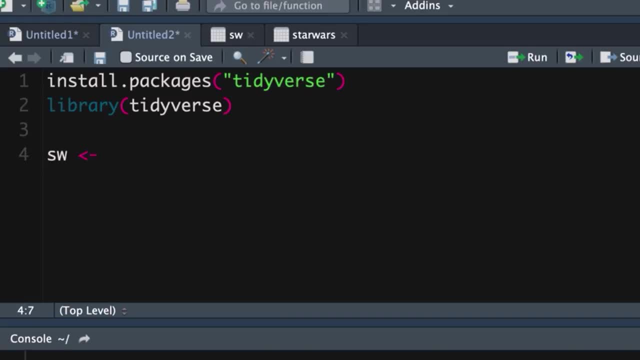 sw and we're going to make that object equal to the Star Wars data set. The first thing we're going to do is we're going to select the variables that we want to work with So we get the pipe operator up and running. shift command m gives you the pipe operator enter. Now we type in the command. 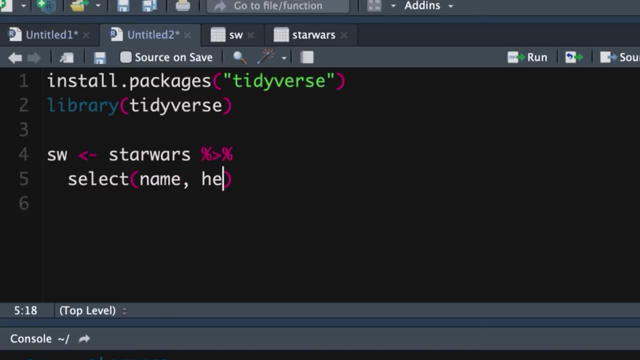 and we're going to add that. So we're going to use the pipe operator and we're going to say height, mass, gender. and which variables do we want? We want name height, mass and gender. Now I'm going to rename mass and call it weight, just because I prefer that. 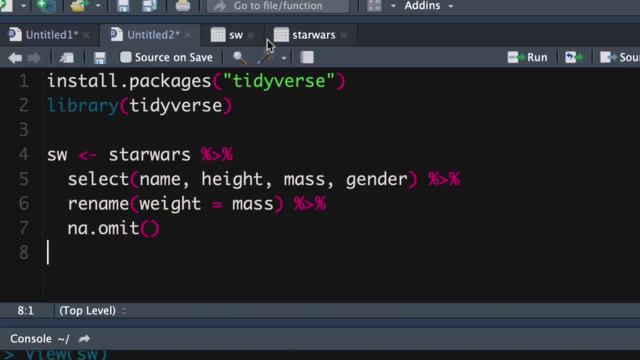 and the other thing I'm going to do is I'm going to get rid of missing values. Voila, missing values are gone. Right, I'm going to create a separate video on how to deal with missing values values some other time. next, i want to take height, which is at the moment in centimeters, and i want 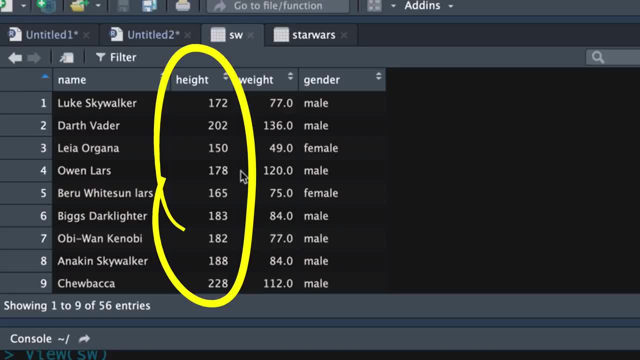 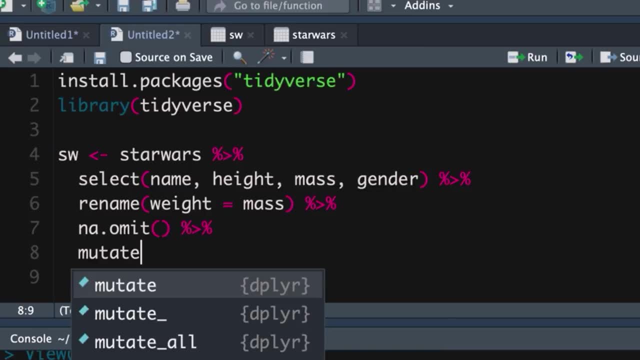 to change that to meters. in other words, i want to divide each of these numbers by a hundred. so i use the function mutate and get a pipe operator mutate, and with mutate you can either create a new variable or change an existing variable. in this case i'm going to change an existing variable. 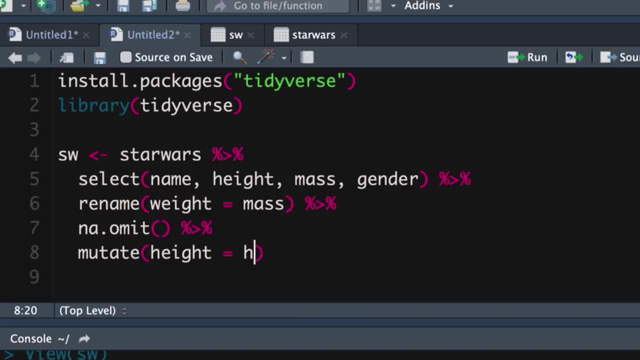 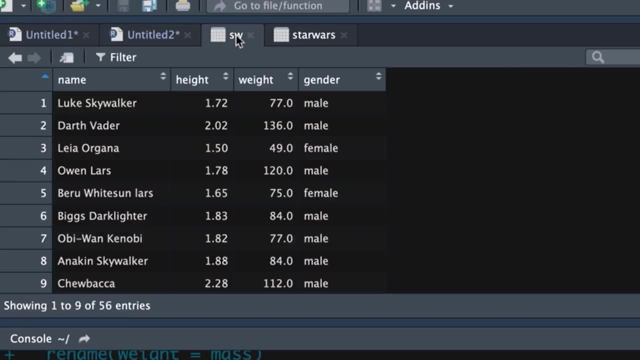 i'm going to take height, make it equal to height divided by 100, and now these are in meters. let's have a look at the gender variable here. we've got it as males and females. we want to change that to m and f, we might. we could change that to zeros and ones- we could. 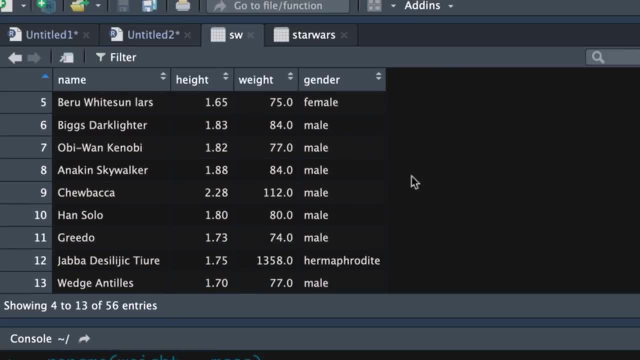 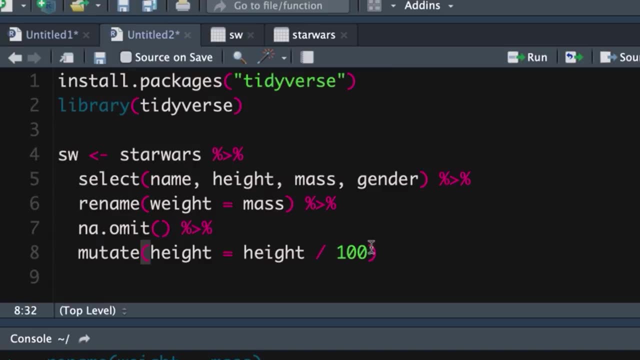 change it to anything we wanted. but importantly, in fact, if you scroll down, we can see that there's not just male and female, but we've also got hermaphrodite here. so, before we carry on, we're going to filter this variable and make sure that we've just got males and females. now i'm going to 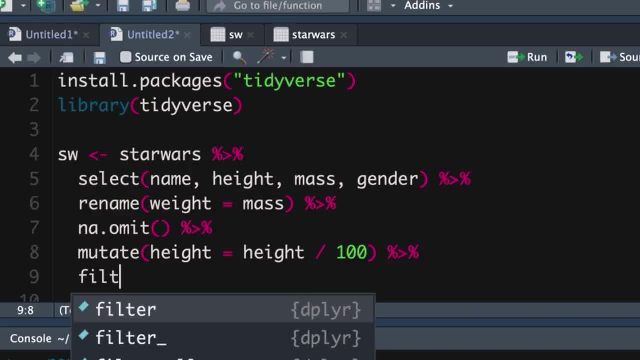 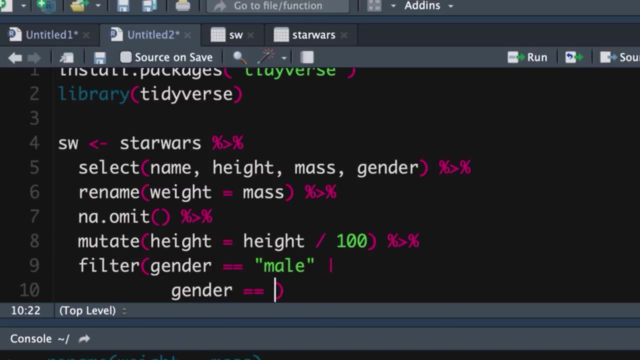 show you two ways to filter. firstly, we can say filter gender is equal to male and then a vertical line like that is: or gender is equal to. we use the double equal signs because we're asking a question of the filter. we're saying: is n equal to n or is n equal to n, or is n equal to n or is n. 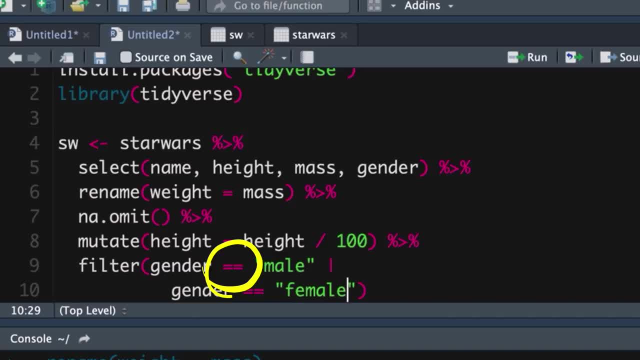 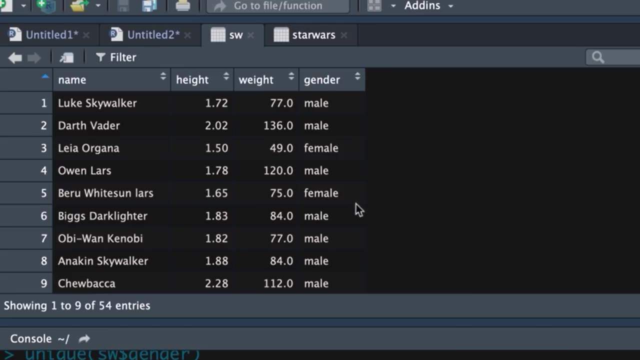 given observation equal to male or is it equal to female and if so, use that observation right. if we use just a single equal sign, that means we're making a statement that this is equal to that push command enter. and now, if we go up into our data set, we don't have anything except males. 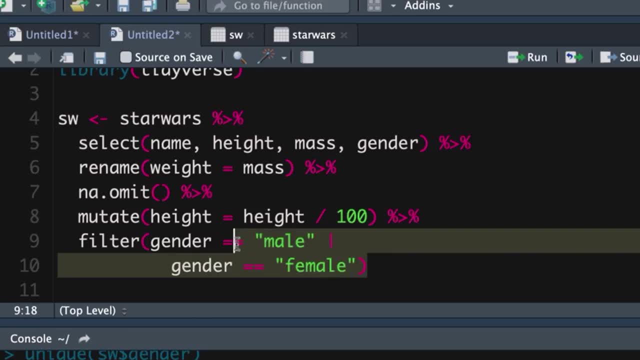 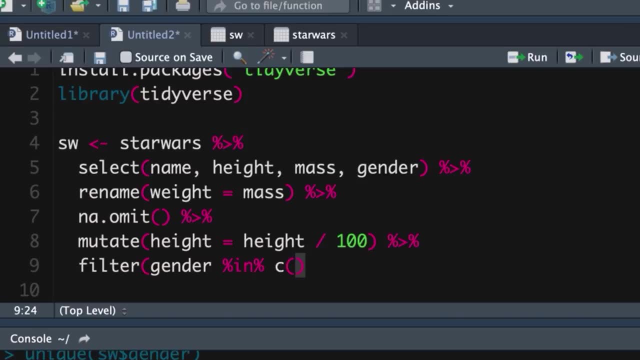 and females. now a slightly more elegant way of doing the same filter is we could say gender n concatenation- male, female. right, that does the same thing. the reason this is a slightly more elegant solution is because sometimes you may have many, many possible- uh- kinds of observations you want to filter for. 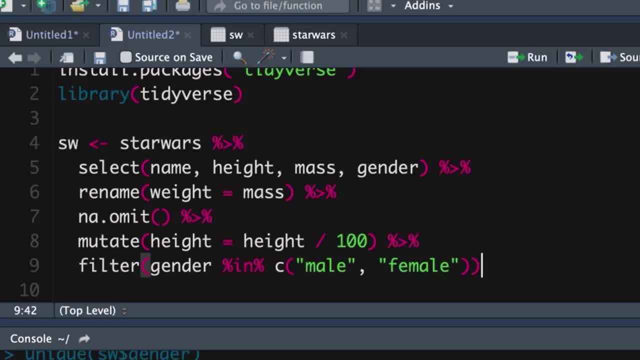 and using a concatenation like that is tremendously useful. okay, so we push enter now and of course, we get the same thing. now let's recode male and female into m and m. so we go, let's do our pipe op. we're going to do a mutate because we're changing an existing variable. we're changing the gender. 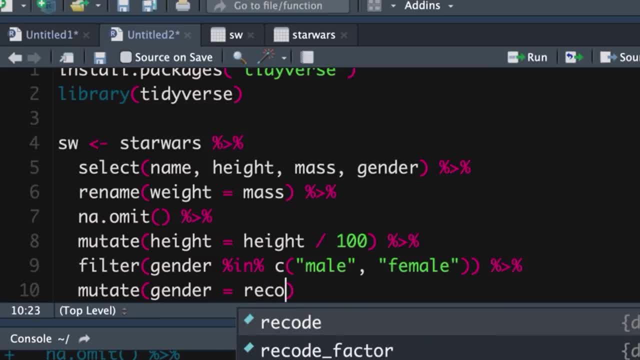 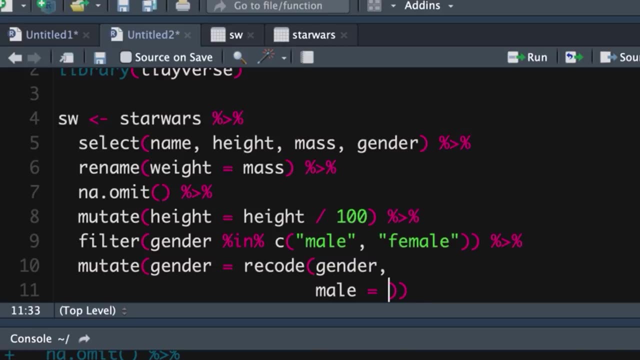 variable it's going to be equal to. we're using a new command called recode, right, and what is it that we're recoding? it's gender. then i like to put a comma just to keep things neat and go to the next line, but you don't have to. we're going to recode male and that's going to be equal to m. 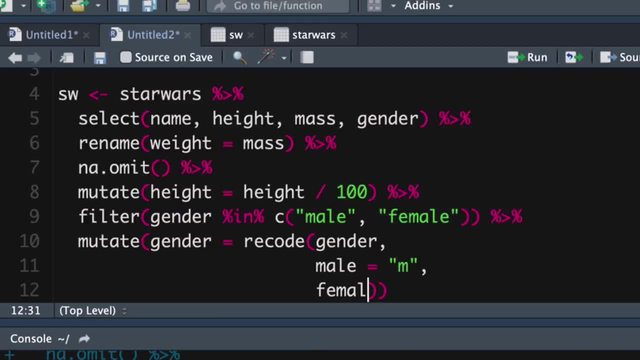 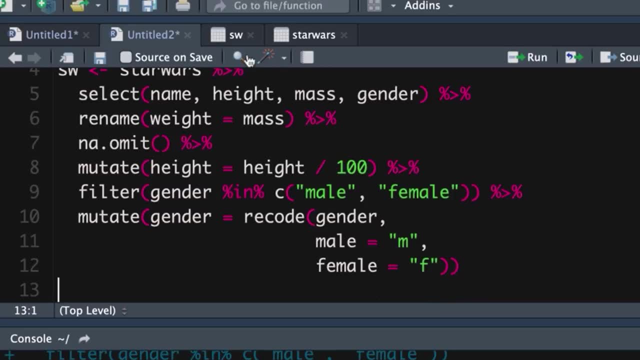 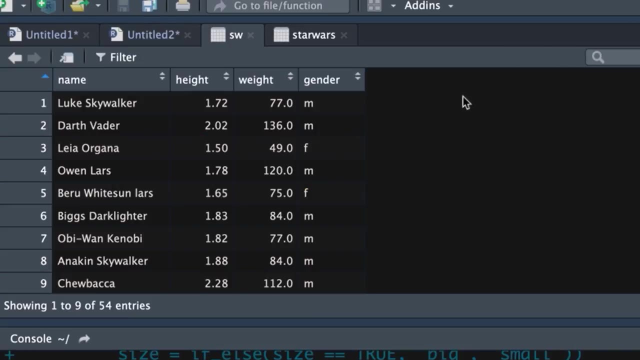 comma, next line. but you don't have to female even before we do any 원래. we're using inc like it's under the c 160, but we're going to use female for this case because we don't know how to maintain the gender. okay, so let's go to the size Ск bound. we want that to be other than 25. 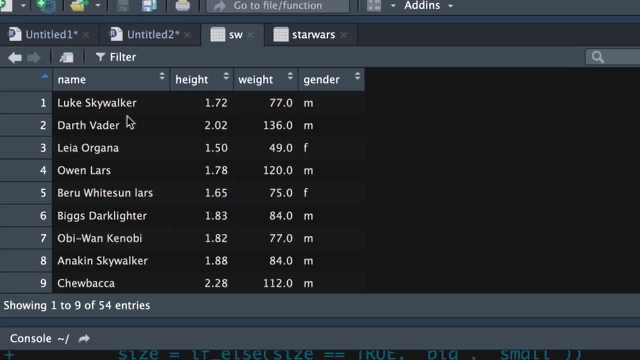 and because we're cutting the side of each first sta, we we just want the first stone here that's gonna be a fishtail for our project to be Locremlin. and then now, like the origin part is name button is the parent. anyway, I'm gonna make it number two. so the first space bar. 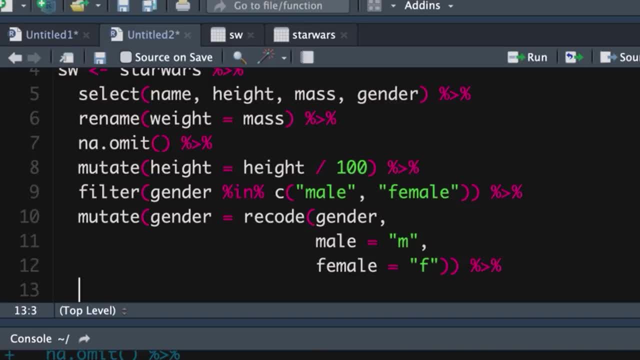 and second. so that's got a set number, okay. and then now, um, we're gonna move this thing over here, operators like saying, and then mutate. we're going to create a new variable called size. it's going to be equal to any observation where the height is more than one meter, and